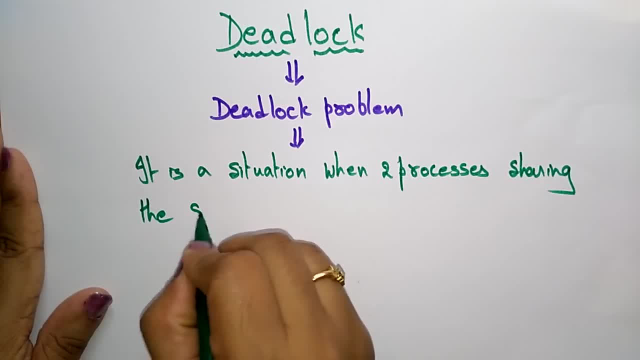 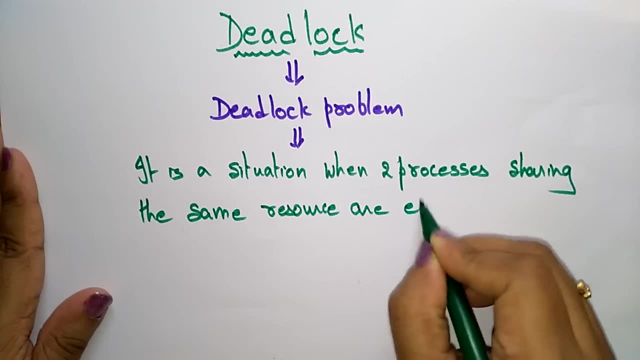 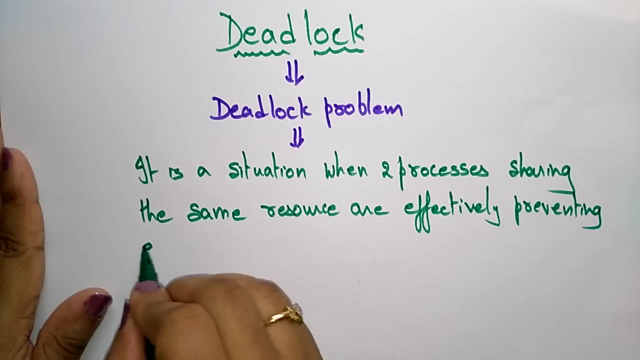 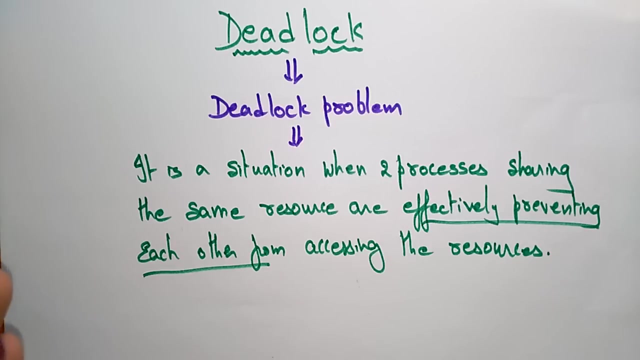 The same resources When two process sharing the same resources or effectively preventing each other each other from accessing the resources. Accessing the resources that you call it as a deadlock. So what is this? sharing the same resources or effectively preventing the each other from accessing the resources? That means- let us take one simple example. 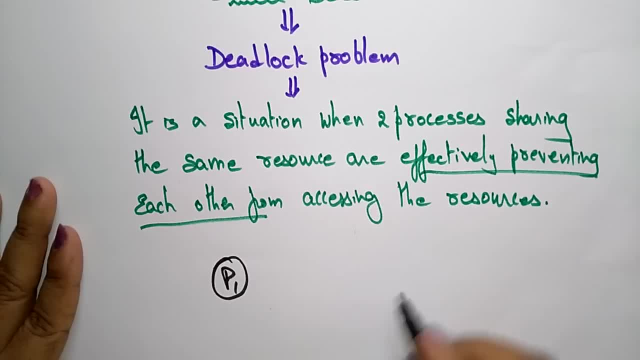 A. P1 is a process and P2 is a process. These are the two process and here R1 is a resource and R2 is another resource. Now P1 is accessing R1 resource. It is already accessing or allocated. R1 resource is already allocated to P1.. But P1 is requesting R2 resources. 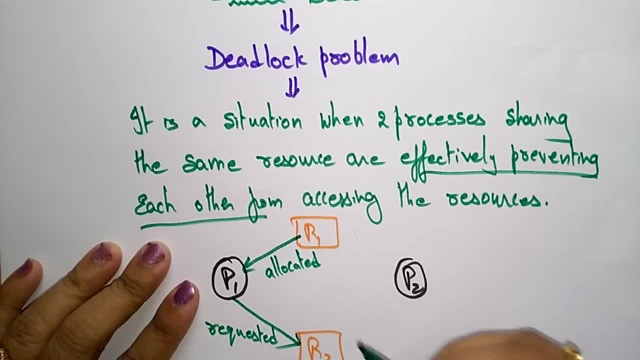 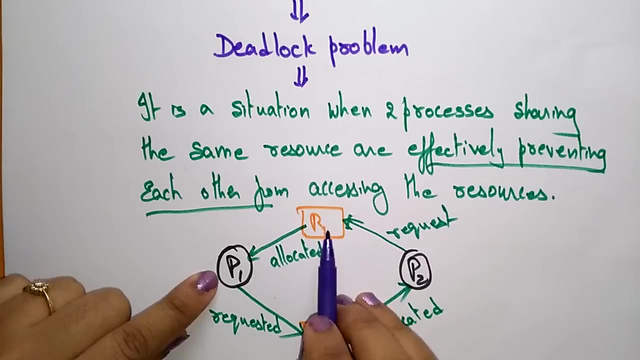 And this side, the P2, is already. R2 resource is already allocated to P2 and P2 is requesting for R1 resource. This state- you call it as a deadlock- What it means. So P1 is already holding R1 and it is requesting R2.. 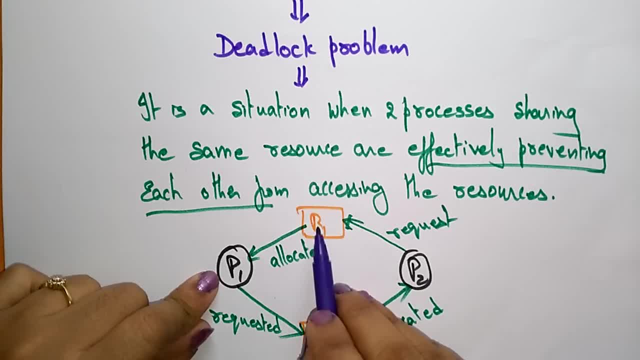 But this R2 is already holding the P2 and it is requesting R1, which is holded by P1.. P1 is holding R1 and P2 is holding R2.. Until P2 releases R2, it does not access. The P1 cannot access. 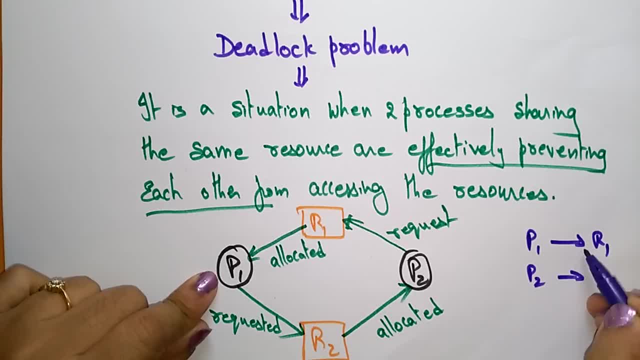 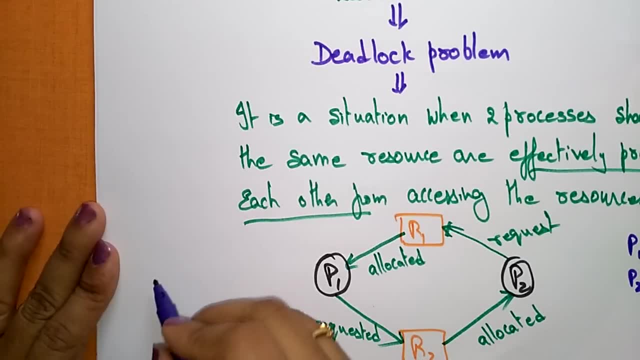 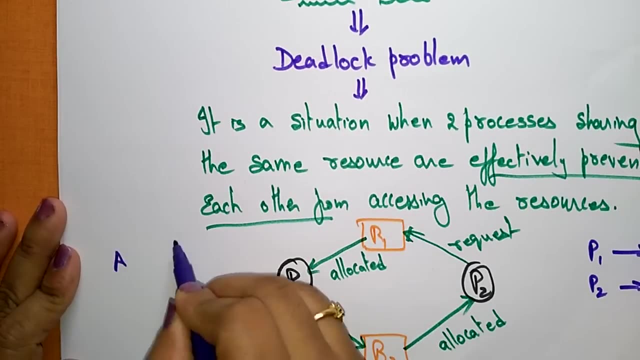 Until P1 releases R2.. Until P1 releases R1, P2 cannot access. So this state, you call it as a deadlock. Okay, Let us take the simple example. A live example Means suppose if you want to call your friend. Okay, A and B, both are the friends. 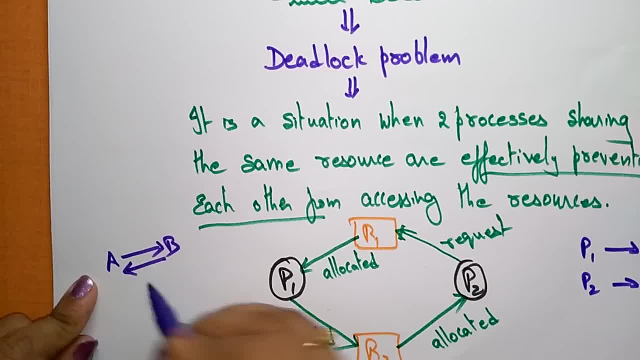 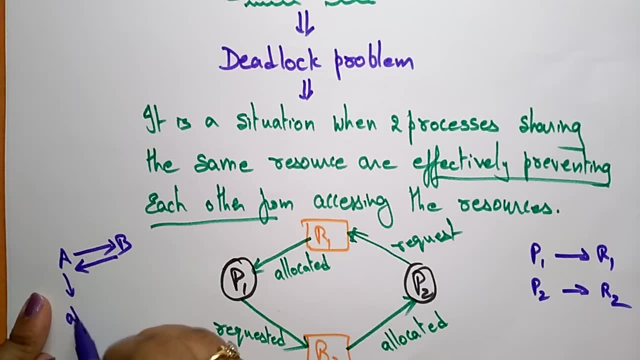 So A wants to call B and B wants to call A. So here A is dialing at the same time, At same time, And B is also dialing at the same time. So then both the persons will become engaged. 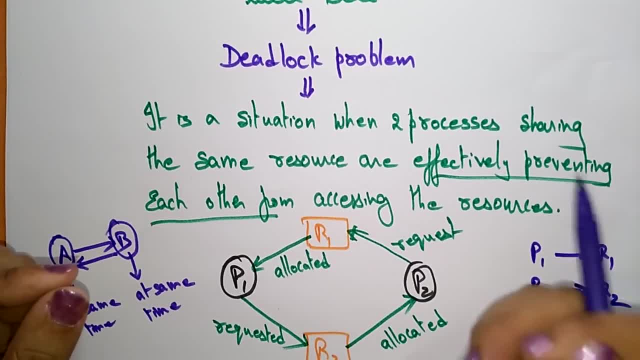 So A leave the phone and B also leave the phone. A dials the B's number and B dials the A number, So then both will get the engaged. No one will respond Because both are trying at the same time. That situation you call it as a deadlock. 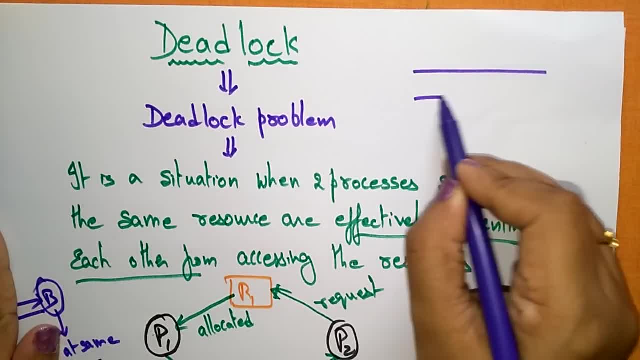 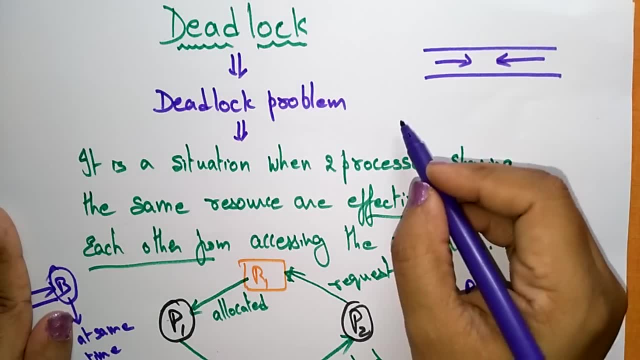 Or else you can take. this is a road. It is a narrow road Here, So one vehicle is coming and another vehicle is also coming in this way. Okay, Now, this vehicle wants to cross this vehicle and this wants to cross this. 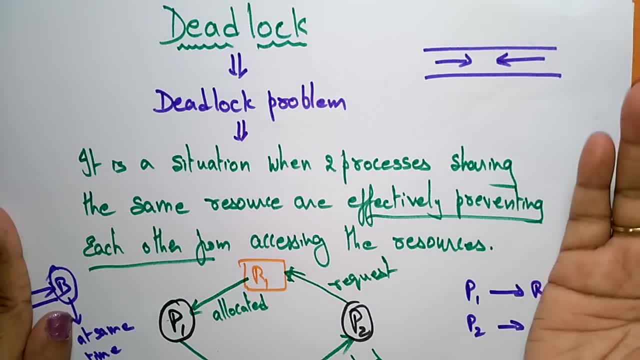 But here there is no space to cross. So what they have to do? So either this vehicle will come back and this will go, Or this has to take a turn and come back and this will go. But they are not ready to go back. 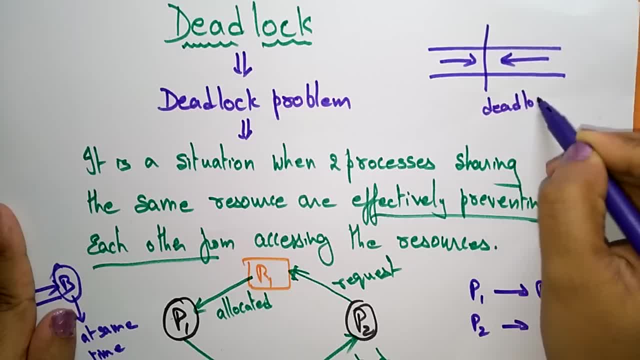 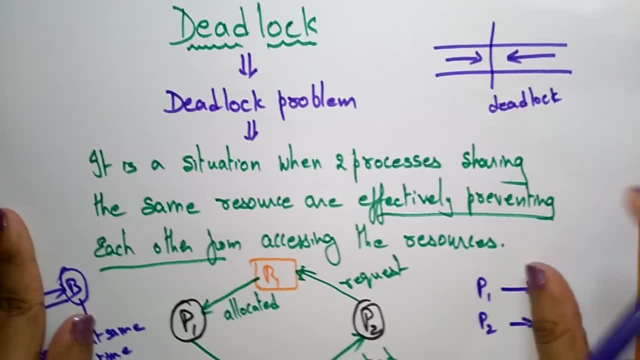 So this state: you call it as a deadlock. Because no one are ready to go, So they want to cross, But there is no space here. So this situation: you call it as a deadlock. So these are the different examples. 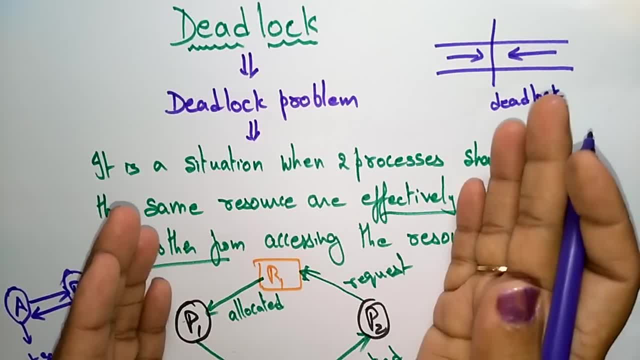 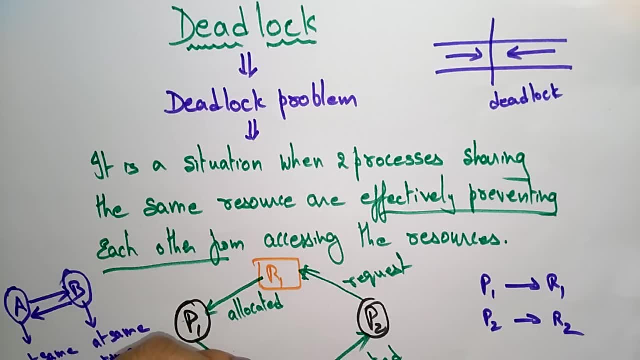 A deadlock means one process is requesting for the resources which is already allocated to other process. Okay, So that you call it as a deadlock state. Until that process is not released, this process has to wait, But that process is not ready to release the lock. 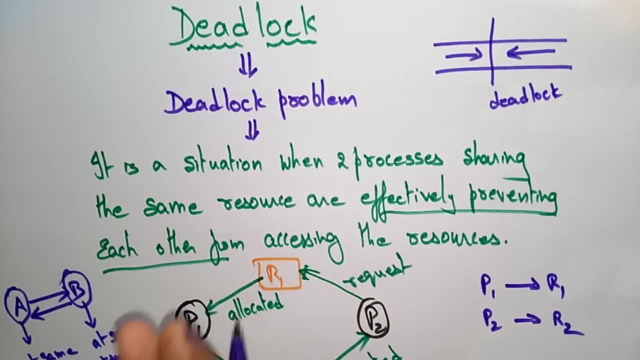 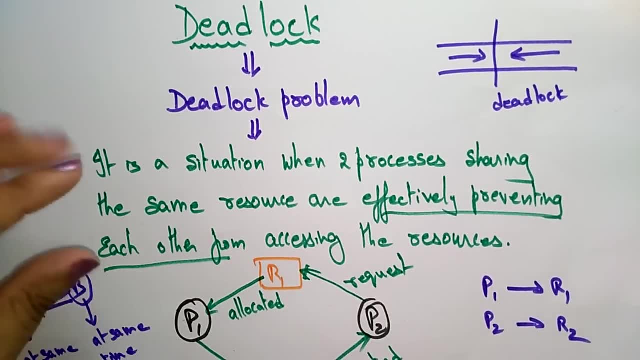 So both are in a wait, So both are in a waiting state. If both the people a process is in waiting state, that state you call it as a deadlock state. So I hope you understand the definition. It is a situation when two process. 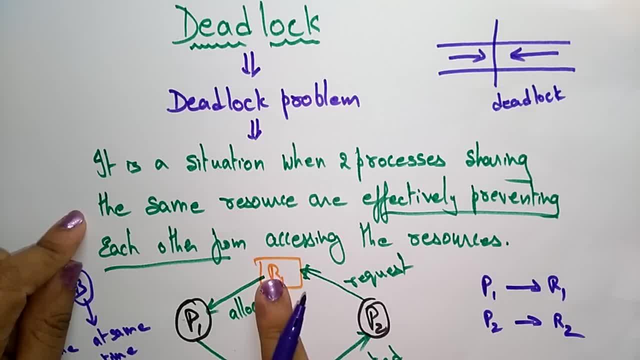 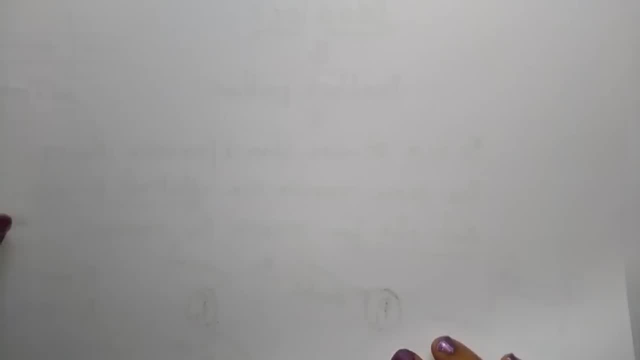 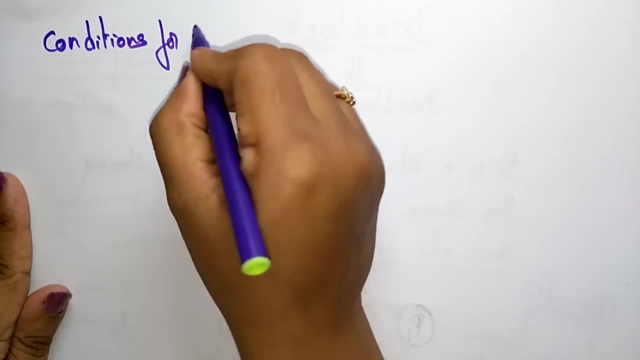 So these are the two process sharing the same resources or effectively preventing each other from accessing the resources. Now let us see the conditions for deadlock. What are the conditions? Conditions, Conditions, Conditions, Conditions, Conditions. It is a happens. 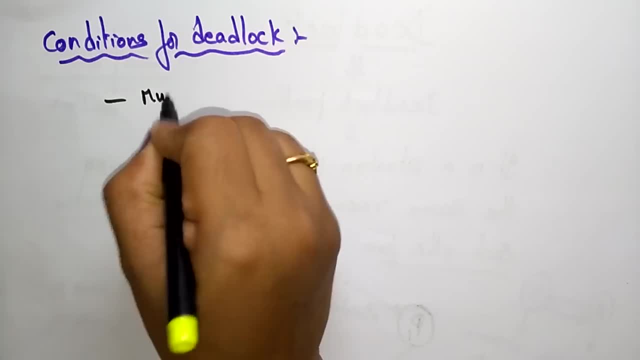 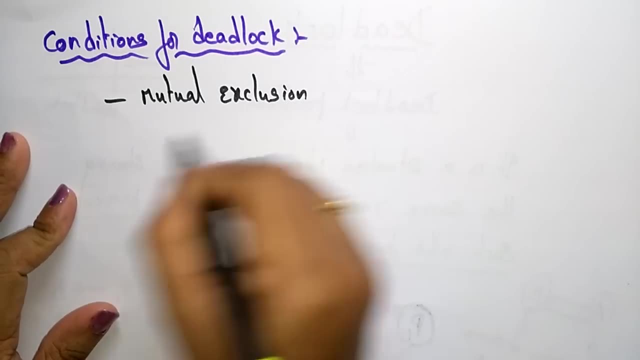 So a person who maybe is having sideline of the order allows his or her hand to be subsidy by just the deep breath as a deadlock. But the other process is saying please don't go with deadlock that what you want, No, no. If so, then the date lock is not guaranteed. 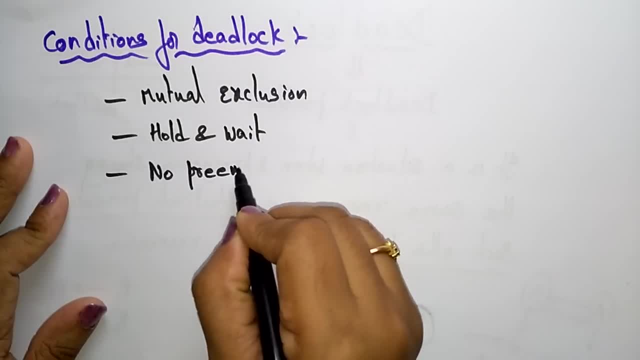 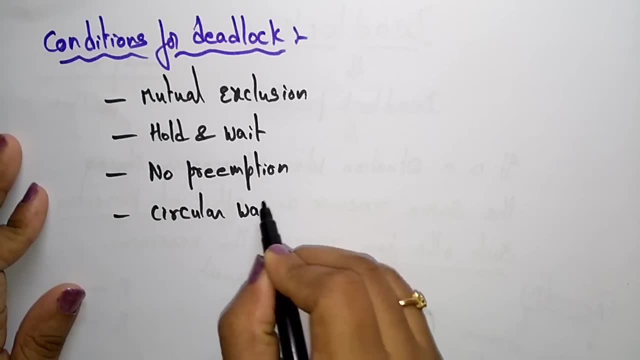 Now let us explain the institution of deadlock: The deadlock. So the deadlock may occur when the process are in mutual exclusion, or when the process is in hold and wait state, Or there is no preemption, or it is a circular weight. the process is in circular weight. so when all these four must, 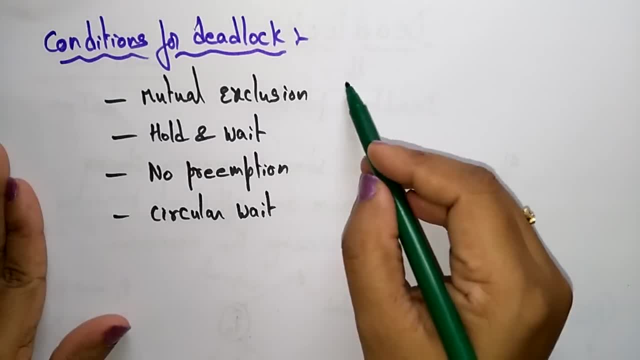 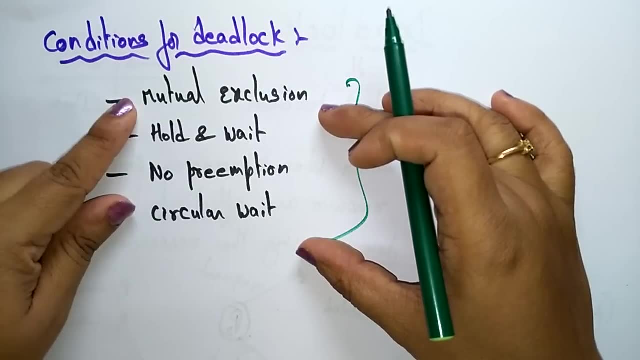 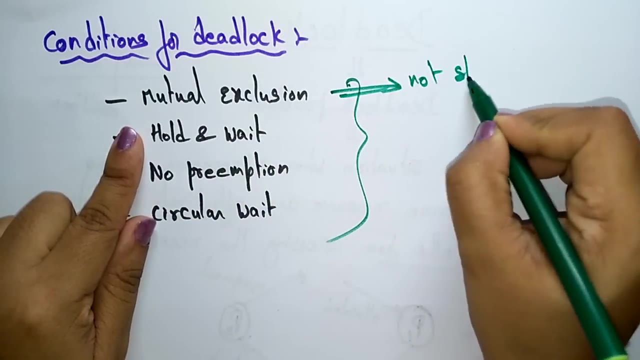 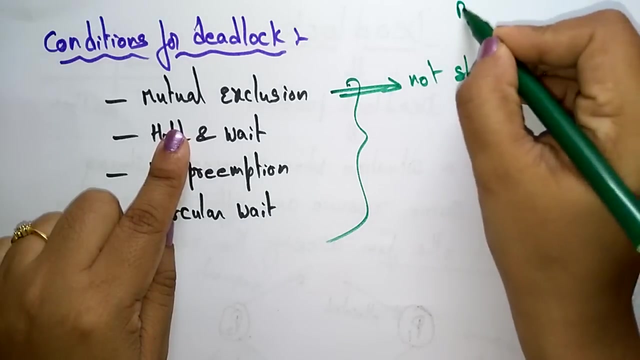 happen simultaneously for a deadlock to occur. so if these all four conditions leads to a deadlock, so mutual exclusion. so mutual exclusion means there is no sharing. mutual exclusion means there is not, it is not shareable. the resources cannot be shareable means the process: suppose R1 resource is there, the P1 cannot, if P1 is accessing and P2 is not supposed to access that. 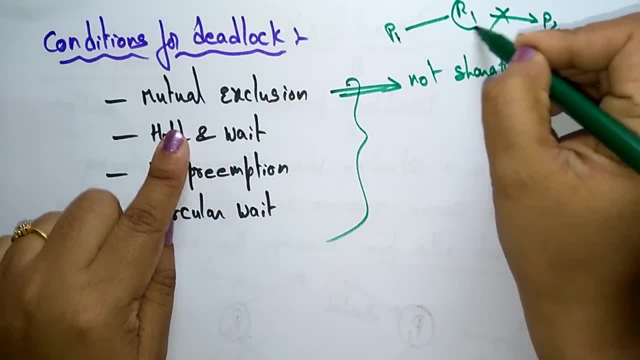 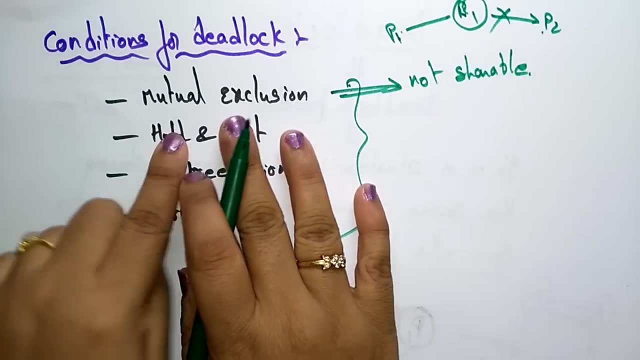 resources. so that is not shareable. suppose if it is, R1 is shareable means P1 can access. at the same time P2 can access and P3 can access if it is shareable. but the mutual exclusion concept means only one process can be shareable. so if P1 is shareable then P2 can access and P3 can access. 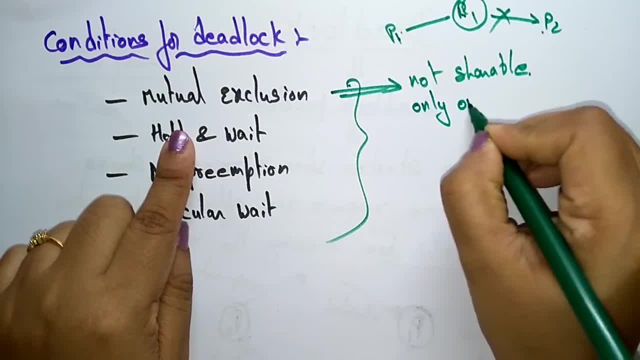 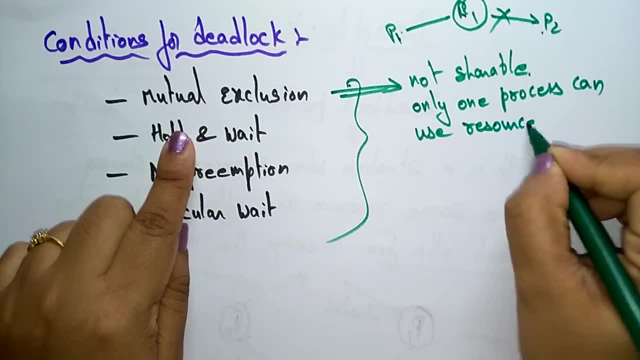 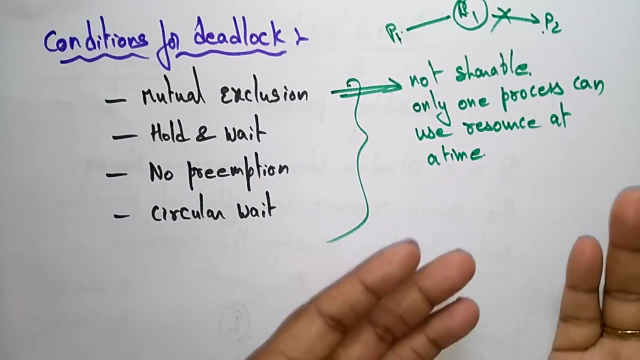 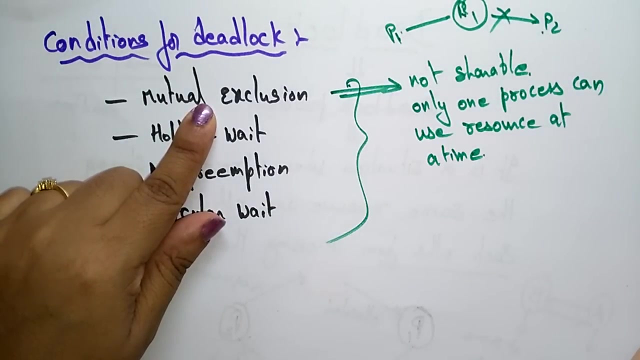 use resource at a time. Only one process can use resource at a time and that process can enter into critical section and execute the work. Mutual exclusion means one by one, One process after that, another process after that. another process means it has to follow the 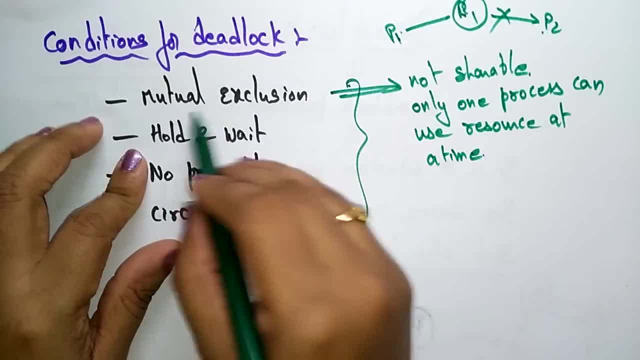 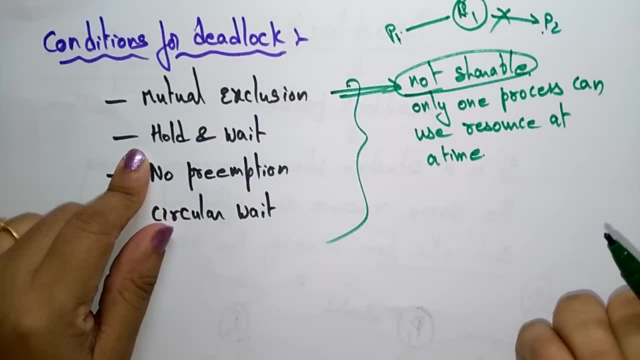 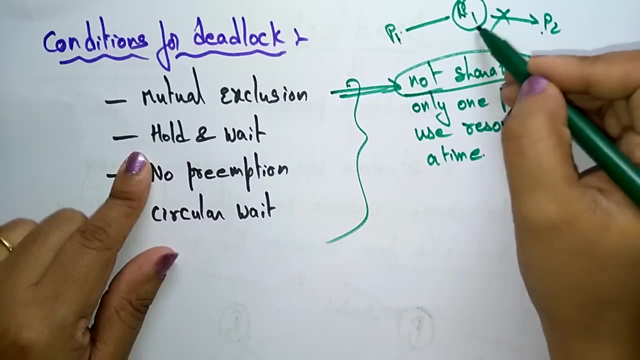 sequence. So the main thing is: mutual exclusion is not a shareable. So if it is not shareable means obviously a deadlock may occur. Means because the P1 wants the R1 resources, P2 wants the R1 resources, every process wants the R1 resources, but that R1 is not shareable. 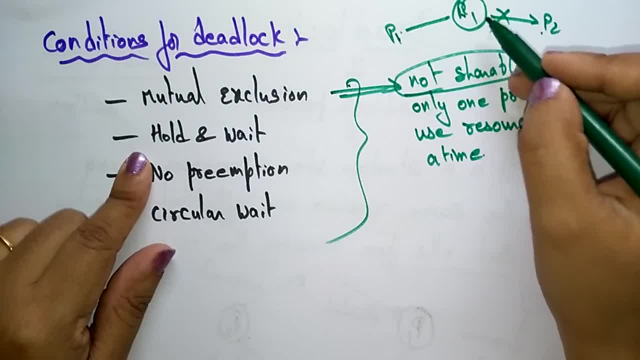 Once the P1 completed, then only P2 can take and P3 can take, but all the process wants to execute at the same time. So that leads to. So if mutual exclusion is not a shareable, then only P2 can take and P3 can take, but all. the process wants to execute at the same time. So if mutual exclusion is not a shareable, then only P2 can take and P3 can take. but all the process wants to execute at the same time. So if mutual exclusion is not a shareable, then only P2 can take and P3 can take. 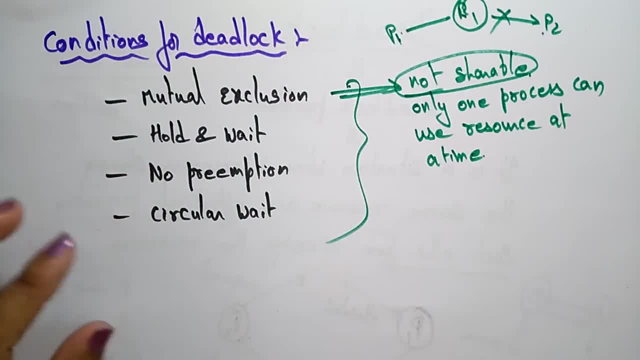 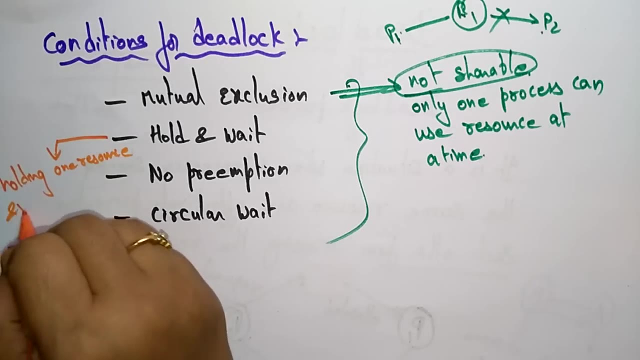 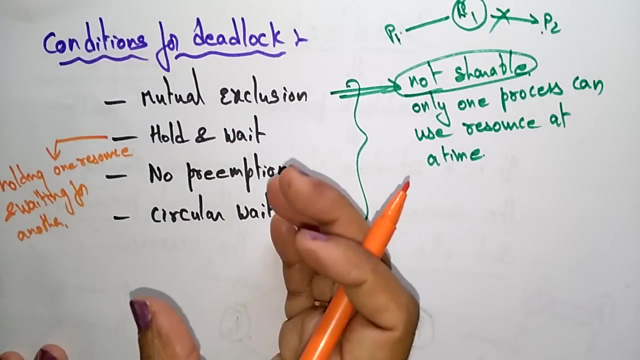 Next, a hold and wait. hold and wait means a process is holding at least one resources and waiting for another. So already that process is holding one resources. it is not not really, even though it is not released, that process is. it is asking for another resources. 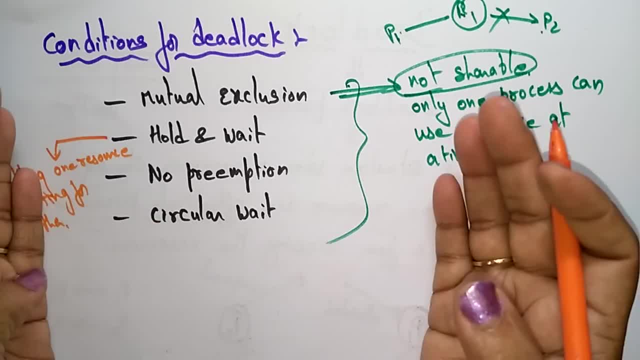 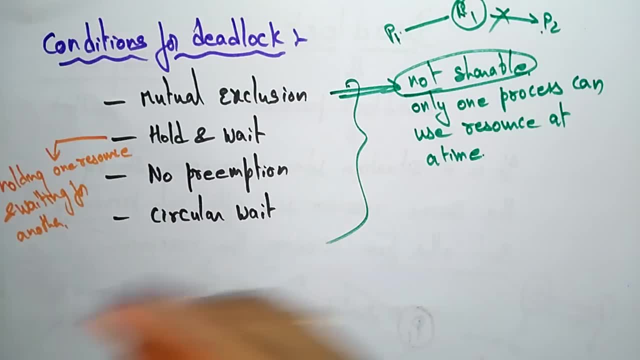 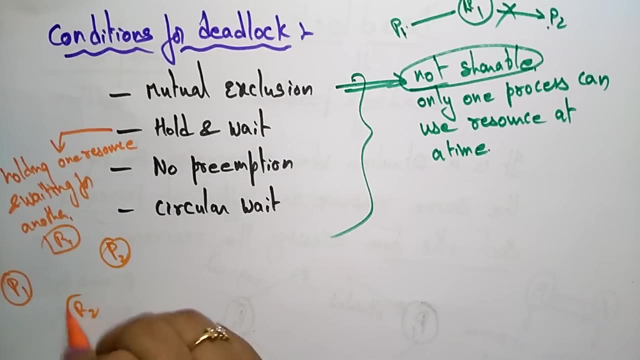 that is, one resource is holding and waiting for another to come, so that case leads to a deadlock. so this is one of the possible condition for deadlock. so that example, what i explained previously, the p1 process, r1, p2, r2- okay, so p1 is requesting for r2 and it is holding r1, so p2 is. 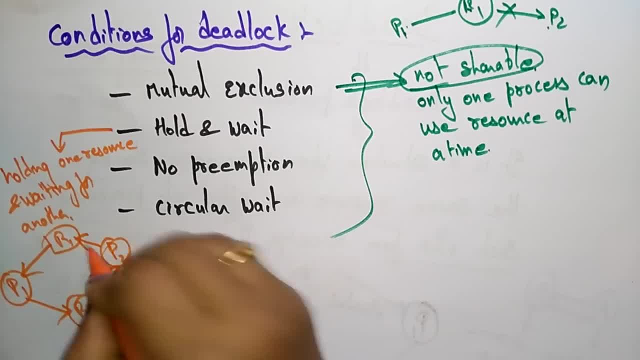 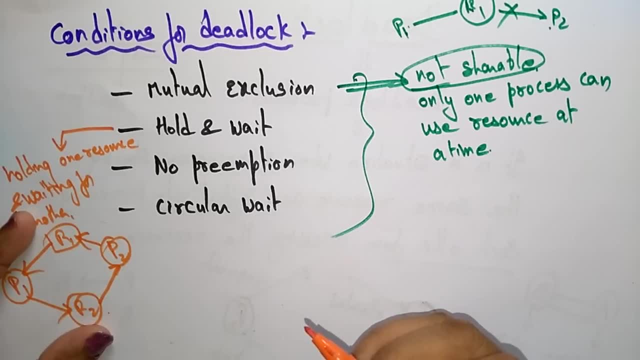 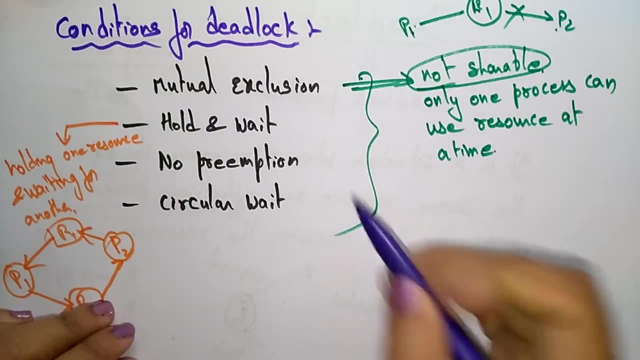 holding r2 and it is requesting for r1. so requesting holding, requesting holding. so this state, you call it as a hold and wait, so this leads to a deadlock condition. now coming to non pre, no preemption, so what you call this, no preemption. so preemption means means if one is 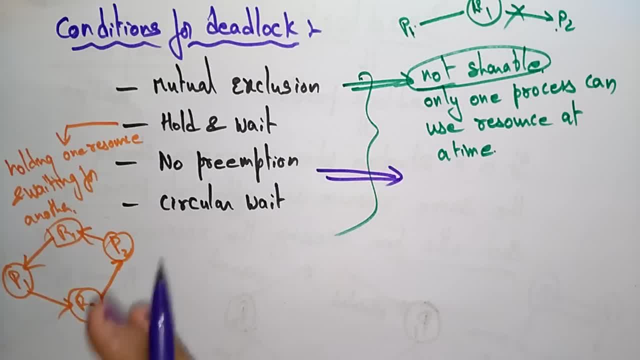 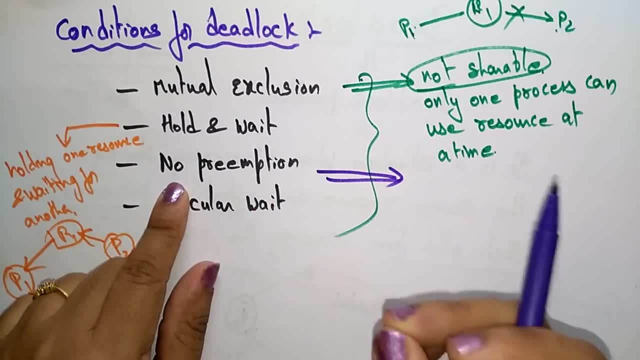 one process completed its work, it can send the resources back so that another process will take you. But here no preemption means a resource, a resources can be released voluntarily by process itself. okay, Only the process can itself release the resources. until that it cannot release the resource. 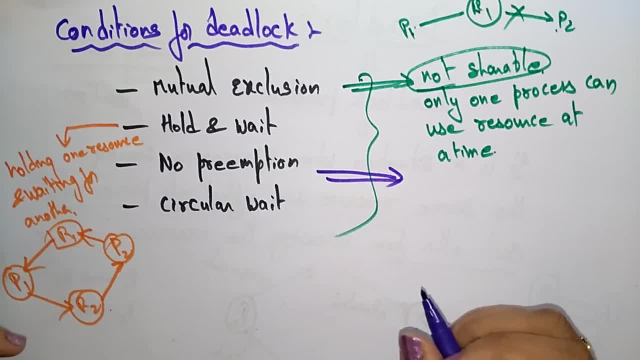 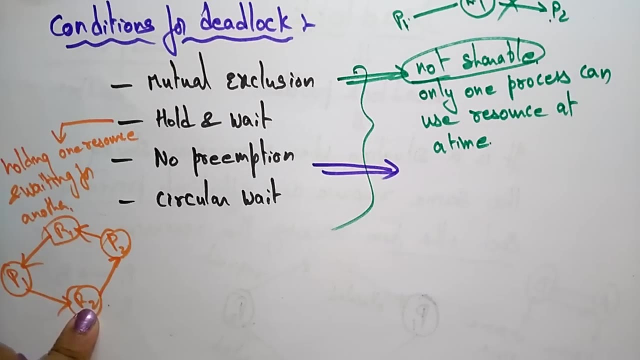 means voluntarily, it can be released, So that you call it as a no preemption Means. suppose P1 acquired some resource. let us take this: P1 acquired some resources and is waiting to acquire another resources. So R1 is already acquired and it is waiting to acquire another resources- R2.. 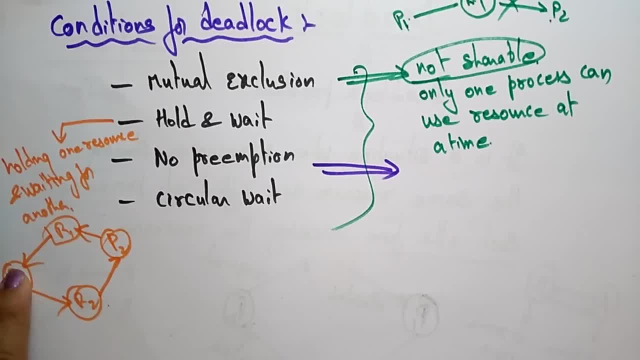 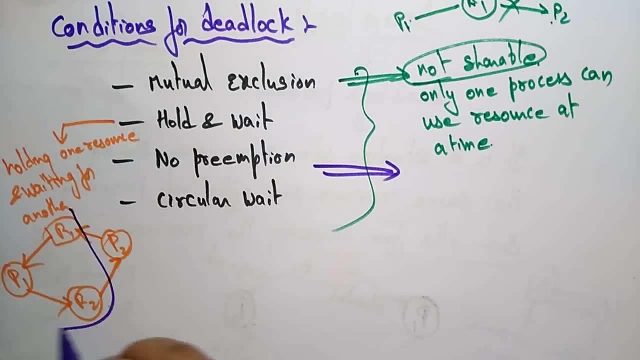 But P1 is not willing to give up this. P1 is not willing to give up R1. So it has already acquired This. state you call it as a preemption. this state you call it as a preemption okay. 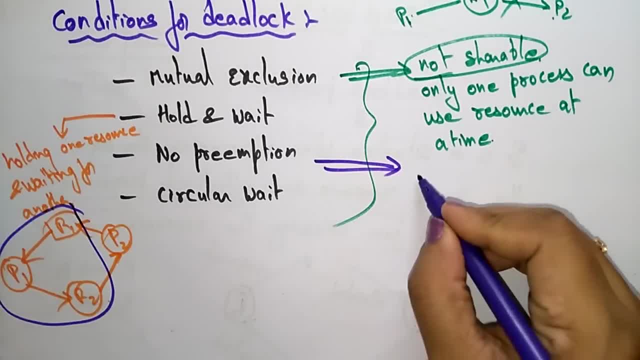 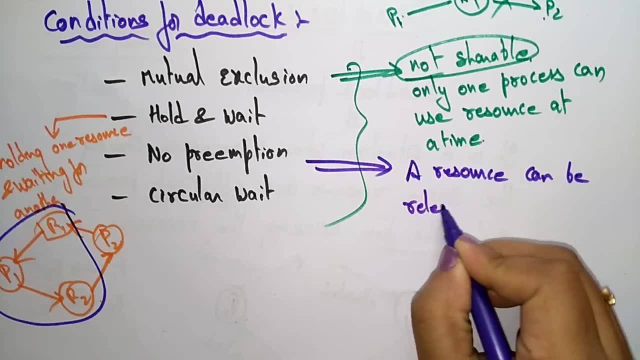 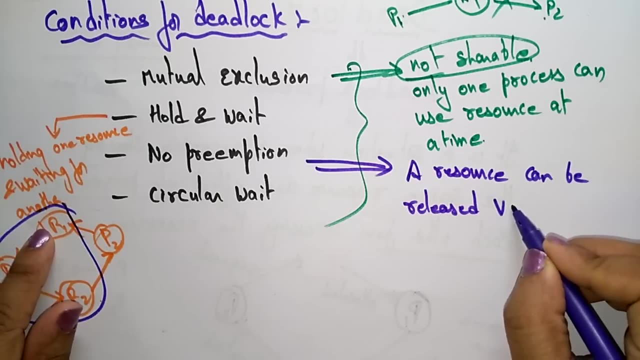 So here what I am saying is let me write that a resources, okay, Can be released voluntarily, So this P1 can voluntarily release the R1, okay, So it has to voluntarily released by process itself. that you call it as a non preemption. 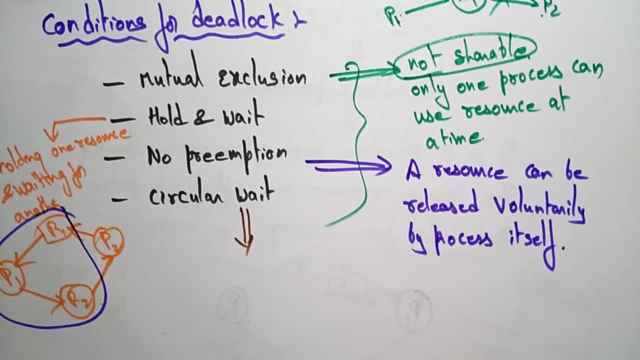 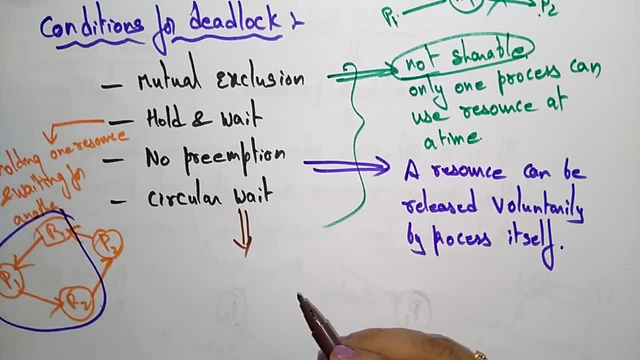 Now, coming to this circular weight. what do you call this circular weight? So this non preemption, no preemption will it leads to the one of the condition for leading to the deadlock, because this P1 is not ready to relieve the R1, but it is asking for R2.. 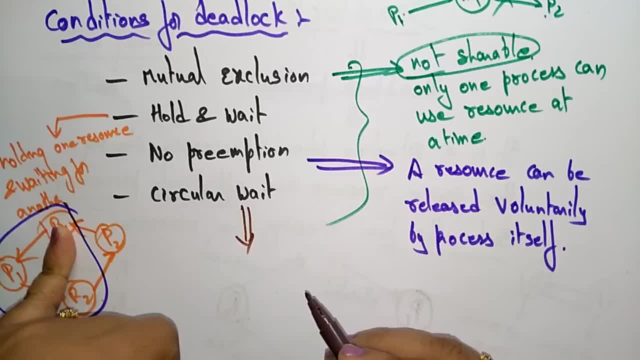 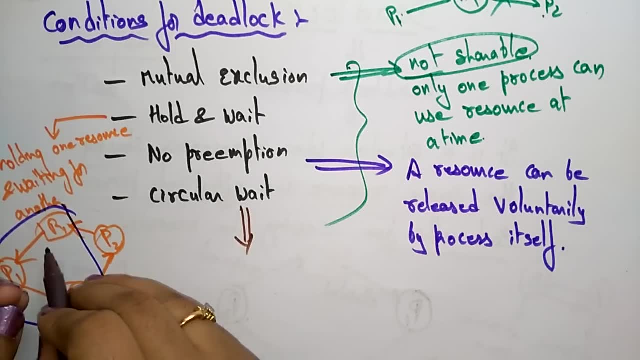 It wants the both the resources- it is not releasing the R1.. Even though its work is completed, it is not releasing the R1. So that is a leads to a deadlock because another process is waiting for R1, okay, So this leads to deadlock condition. 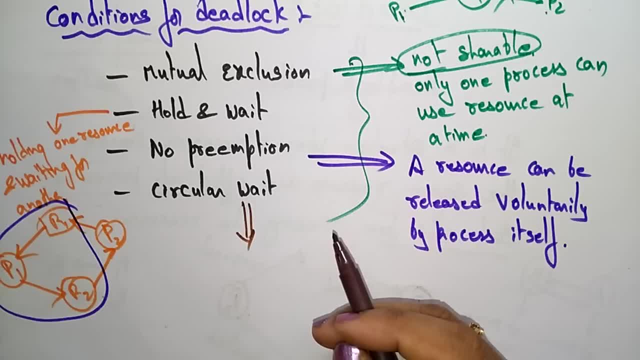 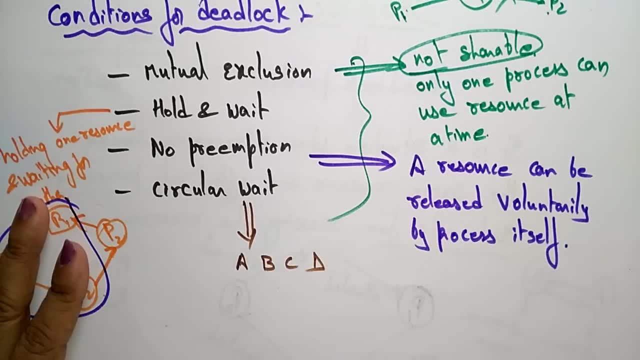 Now coming to circular weight. So what is the circular weight? A circular weight. let us take four process: A, B, C, D. Let us take the four process. So here, the process A acquired some resources, which is needed by B. 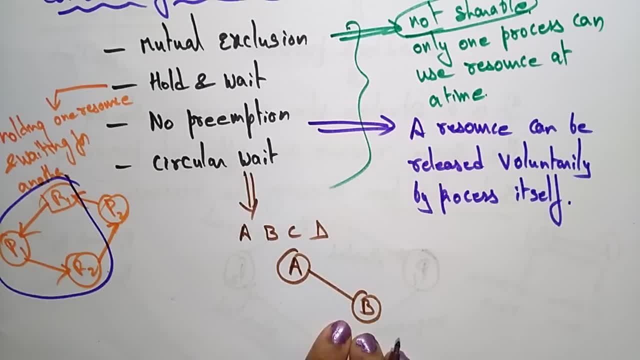 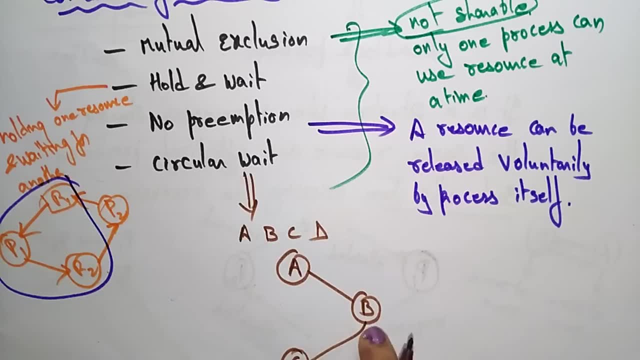 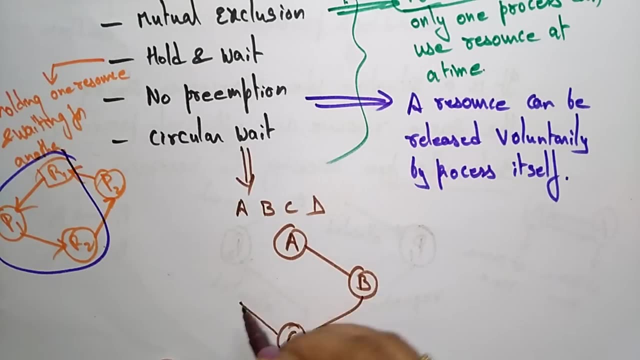 A acquired some resources which is needed by B, And the B acquired some resources which is needed by C. B acquired some resources which is needed by C. At the same time, the C acquired some resources which is needed by D, and the D is also acquired some resources which is needed by A. Here everyone 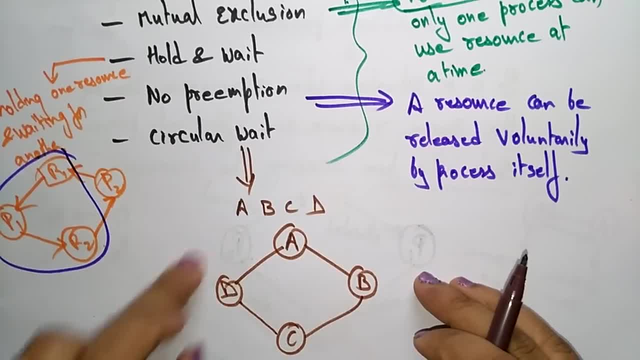 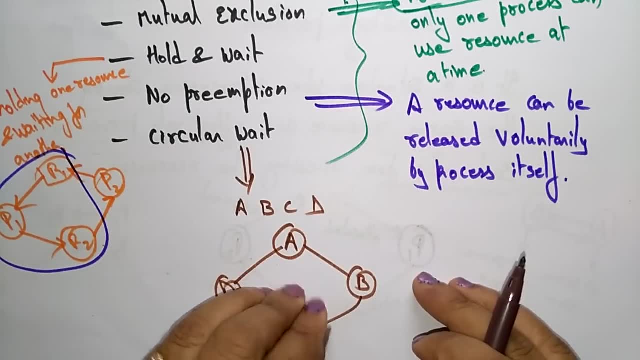 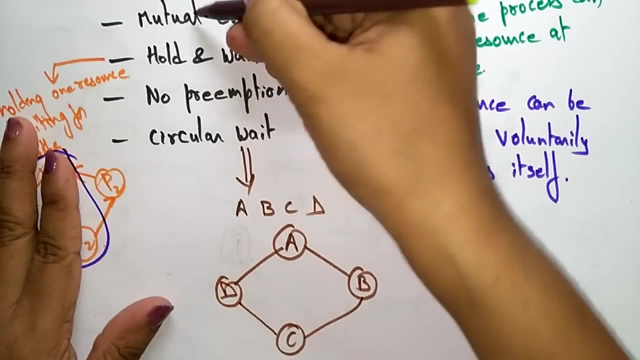 is waiting for another thing. So this condition is- you call it as a circular weight- means there is no solution for this, a deadlock state, it leads to a deadlock. So this condition, you call it as circular weight. So if we prevent any one of this condition, so this mutual exclusion, if you make, 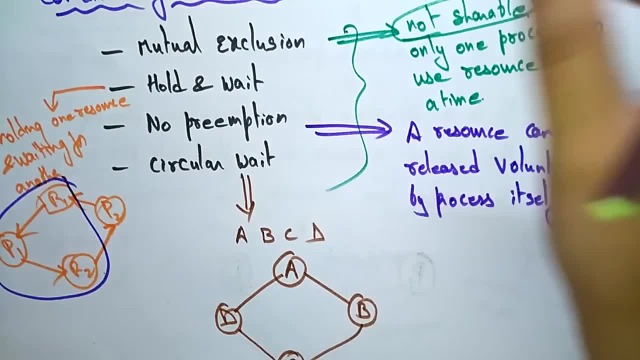 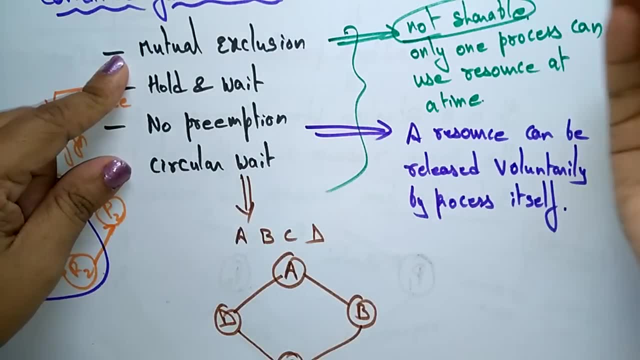 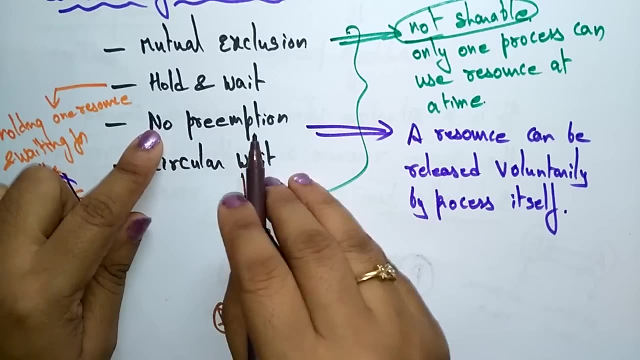 any one of this condition as a false, then you can prevent the deadlock. You can make all the conditions false means you can avoid mutual exclusion by sharing all the resources. You can make the hold and weight as a false statement and you can do no preemption as a preemption.